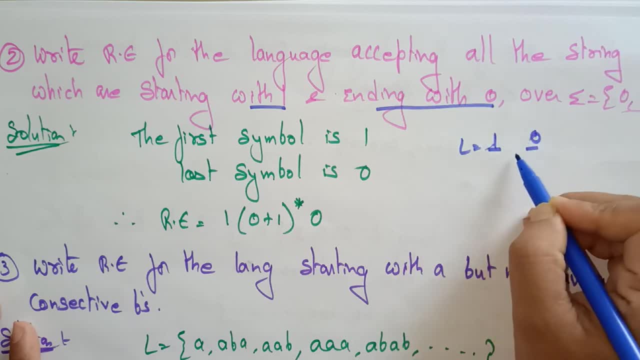 language starts with the one and end with the zero. So in between, whatever the string it can, it can be one, zero or one. whatever it may be. One starts with one and ends with the zero. Start with one and ends with the zero. So whatever it may be, But starting should be one and end. 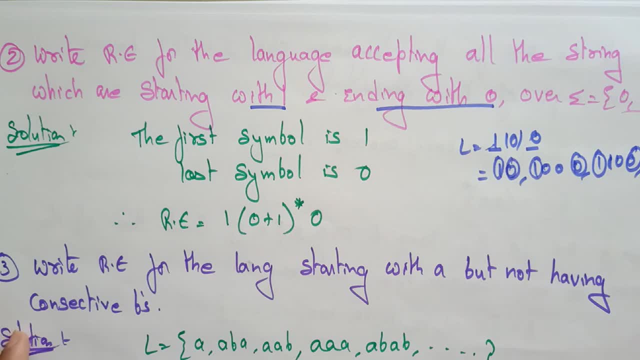 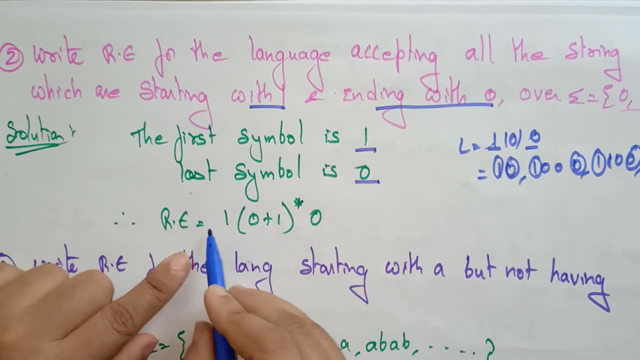 with the zero, Starting one and end with the zero. So this can be represented as the first symbol is starts with one and last symbol is represent with zero. So the regular expression is here: Start with one and end with the zero. So in between, whatever I am taking, that can be represented. 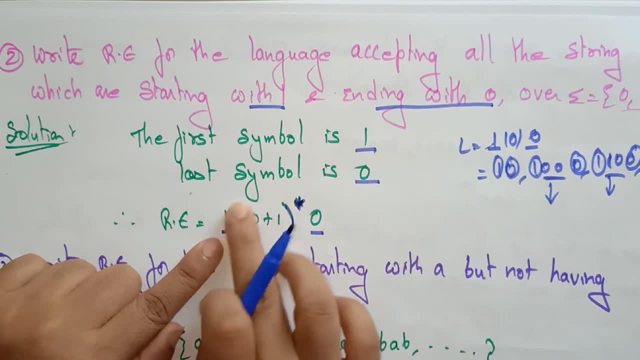 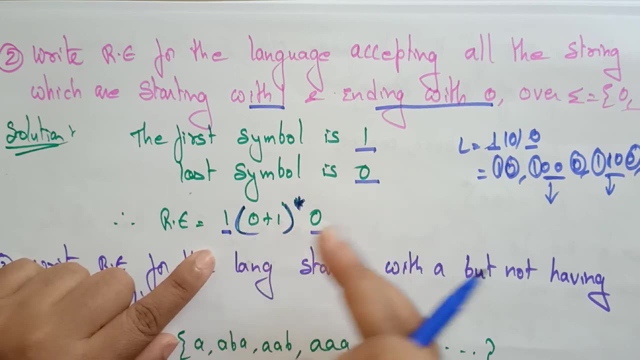 as zero plus one whole star. So in between, whatever it may be the string, either it is 0 or it may be 1 or 0, 0,, 1, 0,, 1, 1, anything, it should be repeated. 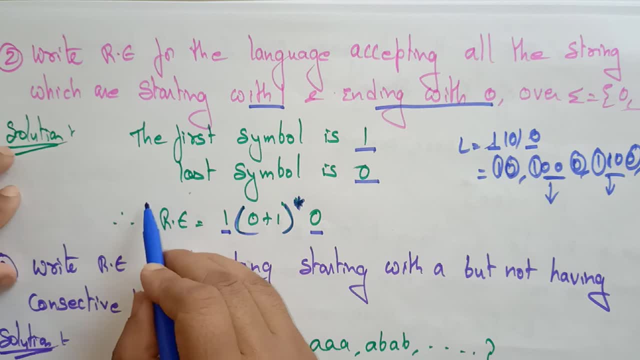 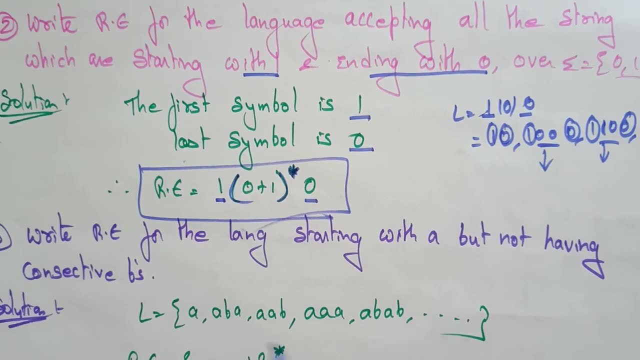 But the string should start with 1 and end with the 0. This is how you are going to represent the regular expression. Next, write a regular expression for the language starting with A. It has to start with A, but not having consecutive B's. 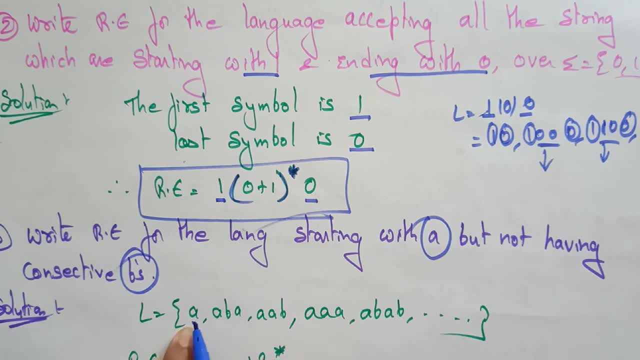 So it has to start with A. This is the language here I have written. Starts with A but not have the consecutive B's Means B B's are not allowed. Whatever B, B, B, B- it's consecutive B's are not allowed. 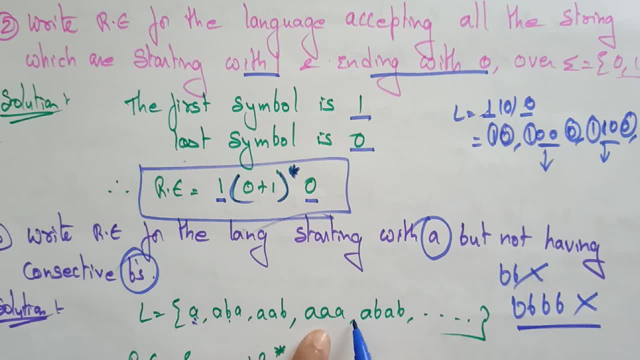 So it may be A or A, B, A A B, A, A, B A B. like this: anything A can be appeared consecutively, but B cannot appear consecutively. So this language can be represented in regular expression like: okay. 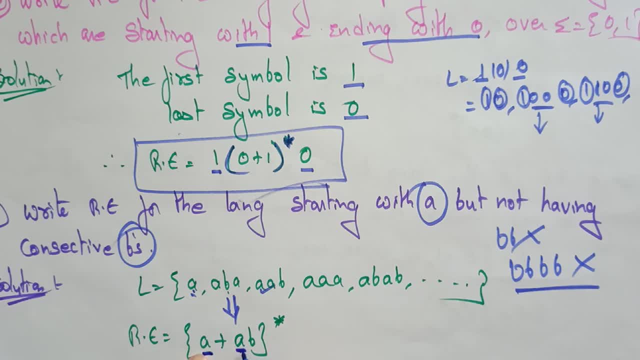 So starts with A, Starts with A, and it should be A B, not A, B, B. okay, You can't write B here. Suppose, if you write B plus A plus A B, it takes the B B also. 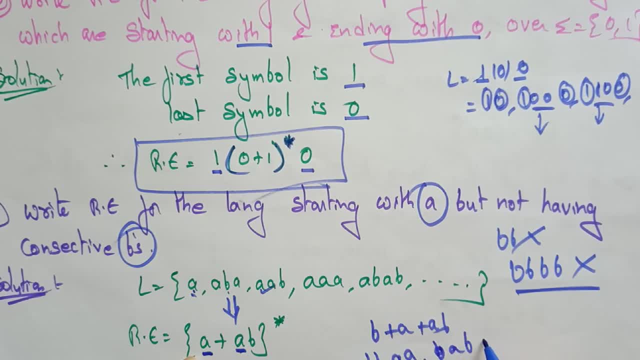 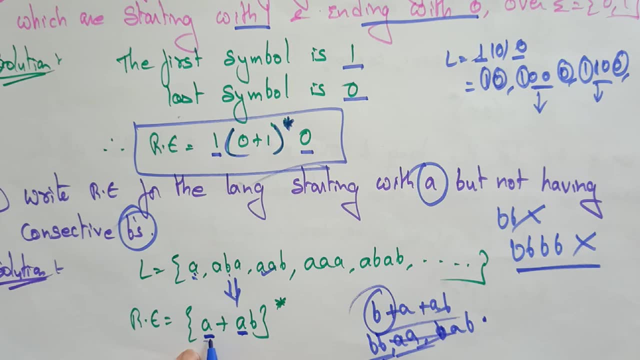 B, B, A, A, B, A, B. so like this: So it can. it can take the consecutive B's also, So don't write B plus, So just write A plus A, B, whole star. 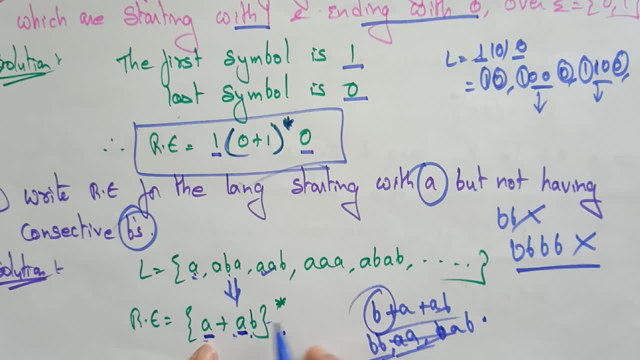 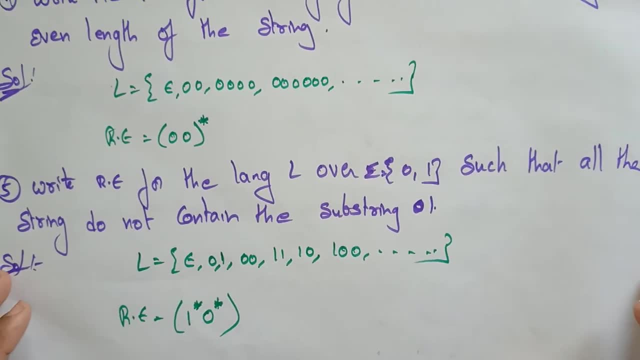 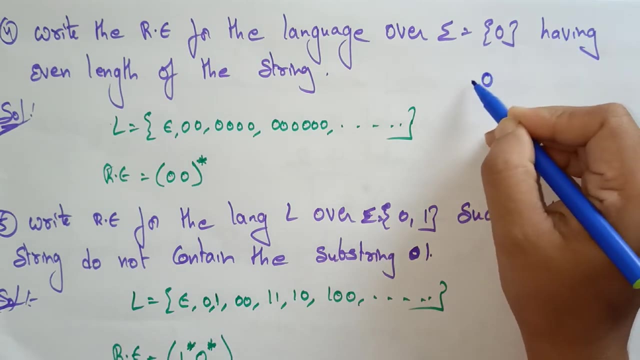 It represents a string that starts with A But not having the consecutive B's. Now let's see the next question. Write the regular expressions for the language over the sigma is equal to 0.. Means only the input string. it's consisting of only 0.